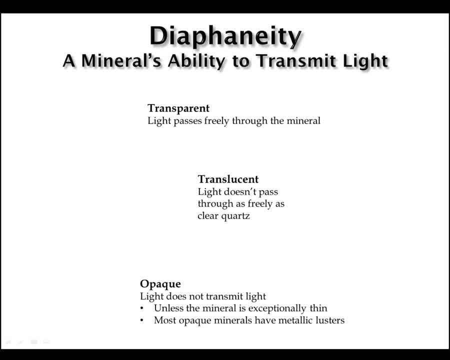 Luster of a mineral is commonly described as being glassy or viscous. Luster of a mineral is commonly described as being glassy or viscous. Diaphaniety refers to the mineral's ability to transmit light. Minerals are commonly described as being either transparent, where light passes freely through the mineral. 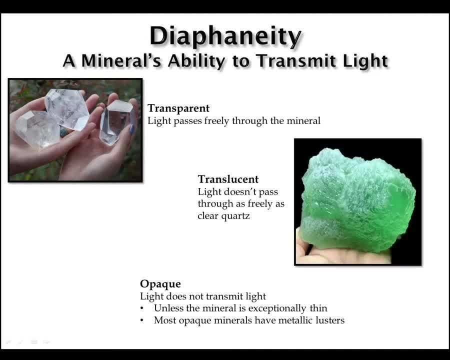 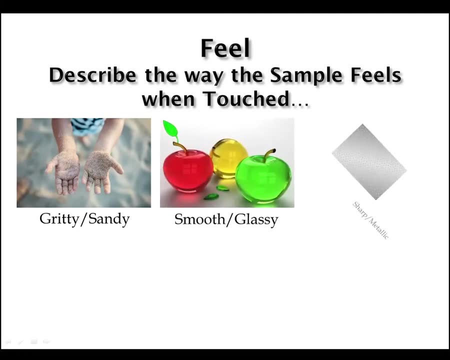 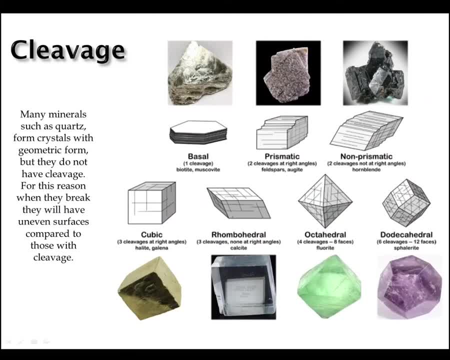 Another tool that can sometimes help to positively identify a mineral is how the mineral feels when it passes through the mineral Cleavage. Cleavage refers to the tendency of a mineral to break along one or more smooth flat surfaces. Many minerals, such as quartz, form crystals with geometric form, but they do not have cleavage. 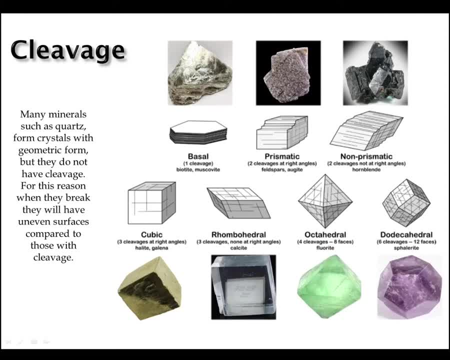 For this reason, when they break, they will have uneven surfaces compared to those with cleavage On a perfect mineral specimen. it is easy to observe cleavage. Simply count how many flat parallel surfaces you can pinpoint. Simply count how many flat parallel surfaces you can pinpoint. 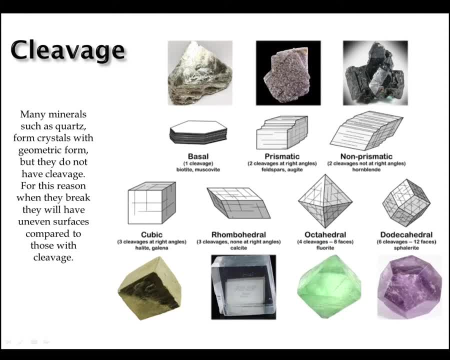 Simply count how many flat parallel surfaces you can pinpoint between your thumb and index finger. We will demonstrate. For the demonstration, we will use arrows. The point of the arrow represents where your thumb and index finger would be placed. Minerals with basal cleavage have only one plane of 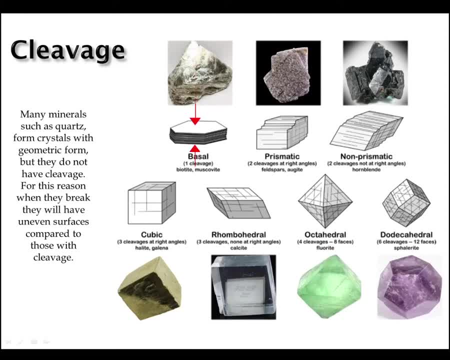 cleavage or only one flat surface that can be pinched between your fingers. Minerals with prismatic or non prismatic cleavage have two planes of cleavage, where one- two flat parallel surfaces can be pinched between your fingers. Minerals with cubic or rhombohedral cleavage have three planes of cleavage. 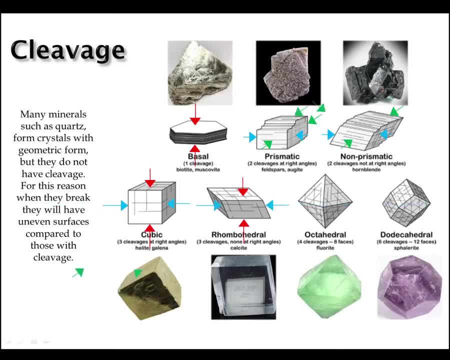 or one, two, three flat parallel surfaces that can be pinched between your fingers. Minerals with octahedral cleavage have four planes of cleavage, or one, two, three, four parallel flat surfaces that can be pinched between your fingers. Minerals with dodecahedral cleavage have six planes of cleavage but will not be. 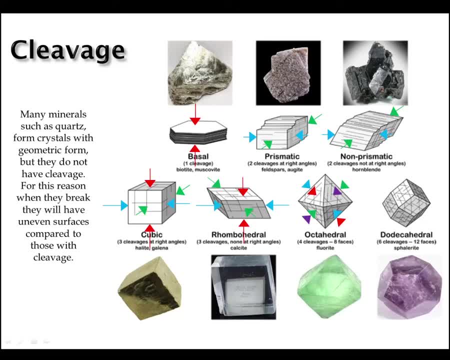 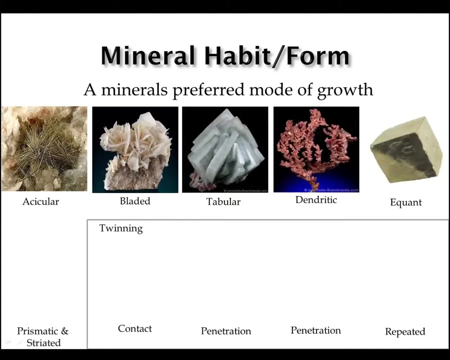 demonstrated here, because it would be visually confusing. Unfortunately it is rare that one is handed a perfect, single crystal of a mineral to identify, let alone crystals large enough to pinch. But practicing with real, perfect mineral crystals can be a lot easier. Mineral habit or form refers to the way a mineral prefers to grow given enough space. 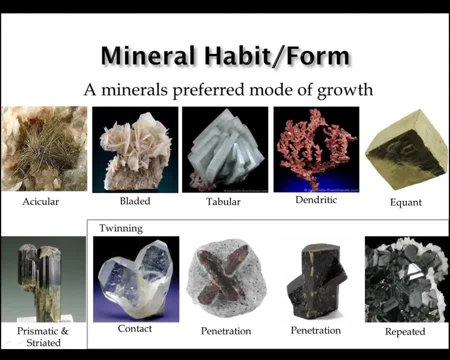 and materials to do so. Many minerals prefer to grow in a needle-like or acicular fashion. Other minerals like to grow in a bladed or tabular arrangement. Some minerals form dendritic or branched-like tree structures. Most of us have seen fool's gold or pyrite, which really likes to grow in the form of a cube. 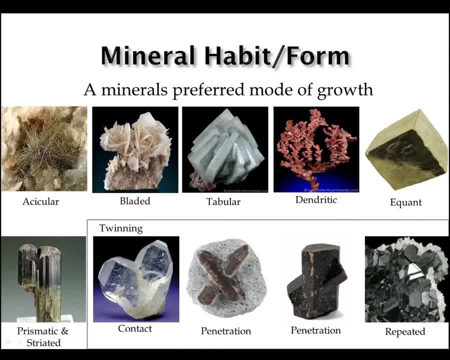 also known as equant. One of my favorites would be a prismatic crystal form with striations or parallel grooves on a surface. Finally, some crystals like to grow within each other. a mineral form referred to as twinning, A mass of minerals, is known as a mineral aggregate, and they 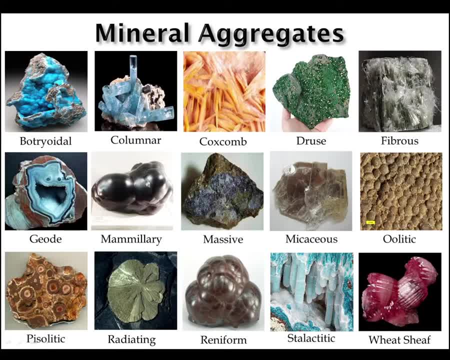 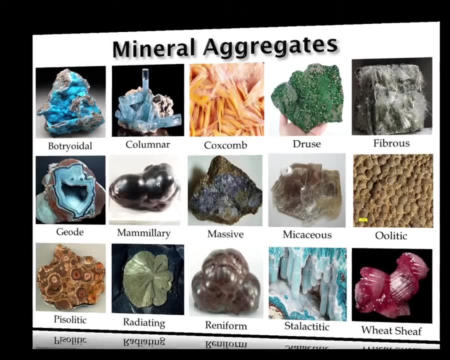 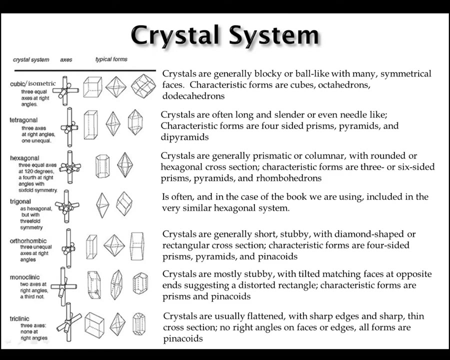 as you can see, can take distinctive forms which all have their own name. This slide shows common mineral aggregates and the respective name designation commonly referred to in mineral descriptions. This is a great graphic to refer back to when identifying minerals. Now I imagine you are thinking: wow, there are so many different crystals with a range of shapes. 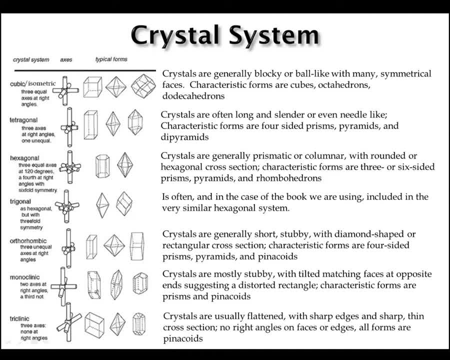 But all minerals actually fall into six basic crystal systems, Because crystals always grow according to simple mathematical laws. The six systems are cubic or isometric, tetragonal, hexagonal, orthorhombic, monoclinic and triclinic. 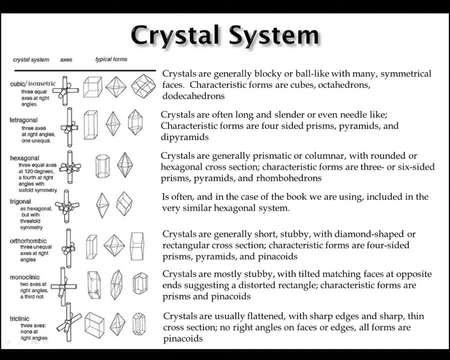 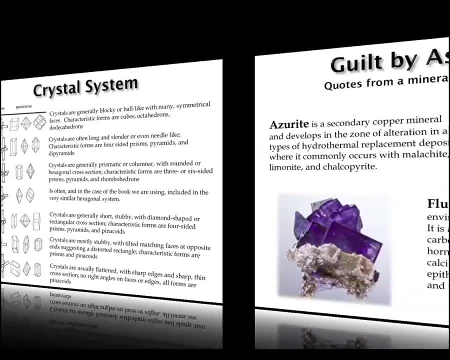 Yes, this slide shows seven crystal systems, but triagonal is commonly grouped with hexagonal. We will not review all of the crystal systems, but we wanted you to know they exist and be able to reference the terminology if needed. The last observable tool is guilt by association. 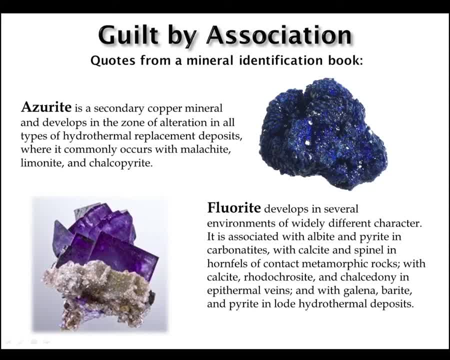 In mineral descriptions, it is common that minerals which are associated with each other are listed. For example, azurite is commonly found with limonite and chalcopyrite, and fluorite is associated with specific suites of minerals in specific geologic environments. 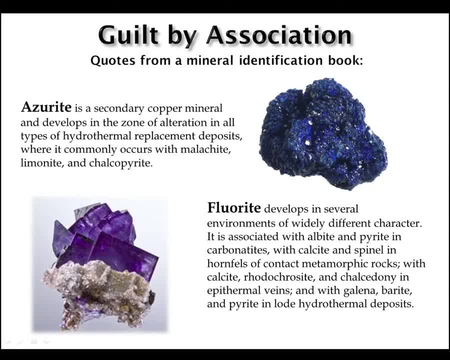 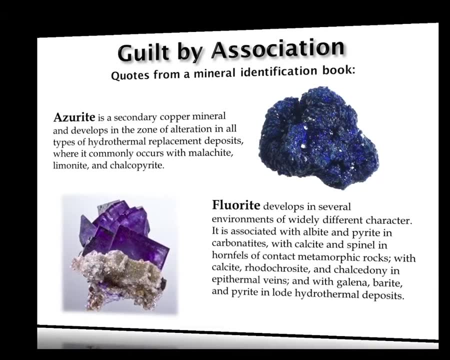 In some cases, when a mineral identifier is stuck between two possible candidates, knowing where the mineral is from and identifying other minerals that may be in the sample can really help with positive identification Guilt by association. Now let us move on to tools we use to test minerals. 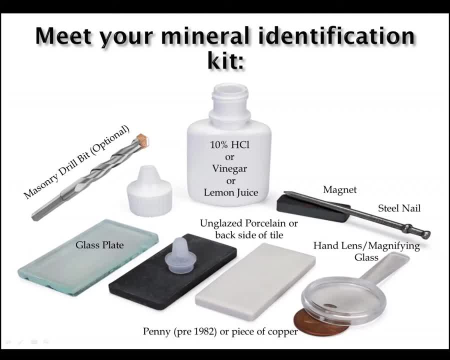 Meet your mineral identification test kit. A basic identification kit consists of some pretty common household items: A magnet, a steel nail, a hand lens or magnifying glass, a piece of copper or a piece of silver. A piece of copper or a piece of silver. 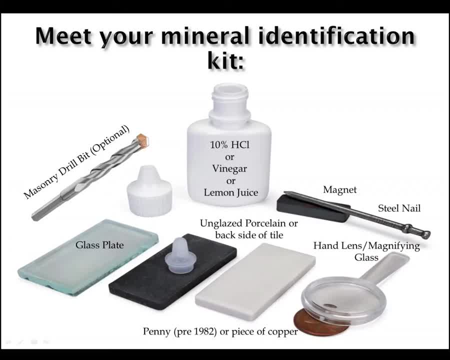 A piece of copper or a piece of silver, A pre-1982 penny, an unglazed porcelain streak plate, a form of weak acid and an optional masonry drill bit. A 10% hydrochloric acid solution works best as the reaction is very visible. 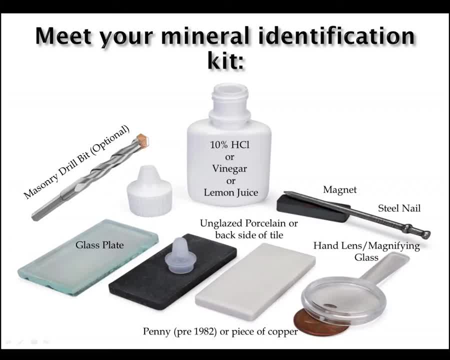 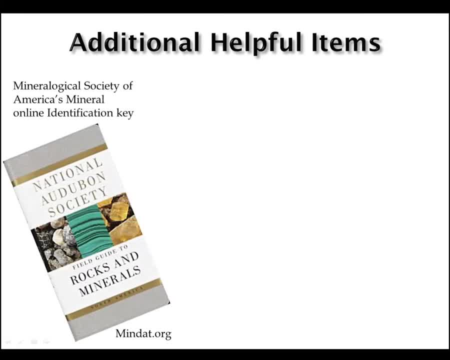 Another method would be to put the sample in a cup of vinegar or lemon juice and see if bubbles start to form and float to the surface. guide for actually identifying the minerals. If you prefer a book, I recommend the National Audubon Society's Rocks and Minerals Identification Guide. It has many minerals and is relatively 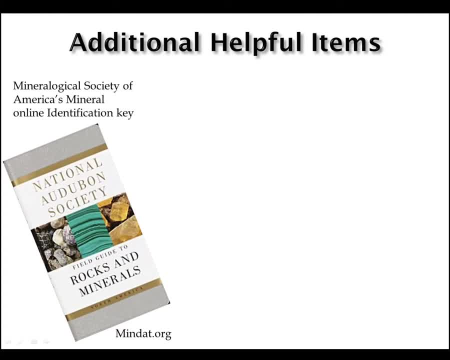 easy to navigate through. We will also be looking at some very helpful websites that are free to use later in this video. A blacklight with shortwave and longwave capabilities is handy but not necessary, And if you really want to get into mineral identification and 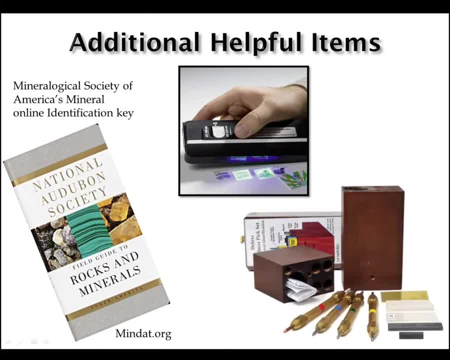 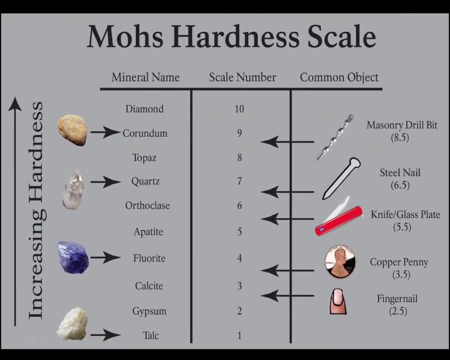 want to be more precise on your hardness test, which we will talk about next. the Deluxe Hardness Pick Set for Mineral Identification is really handy but not cheap. So what do we do with all of these tools? Well, we perform tests on the minerals One. 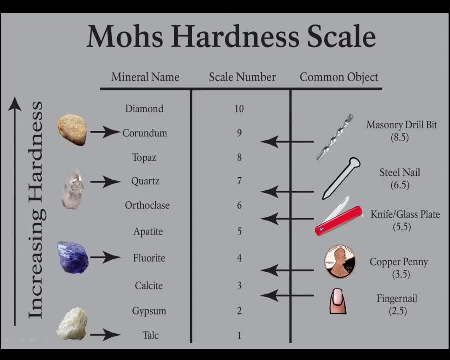 of the most important tests is to see if the minerals are in the right condition. If the minerals are in the right condition, you have to make sure they are in the right condition, and this is what we do. The first test is called a mineral hardness. Each mineral has 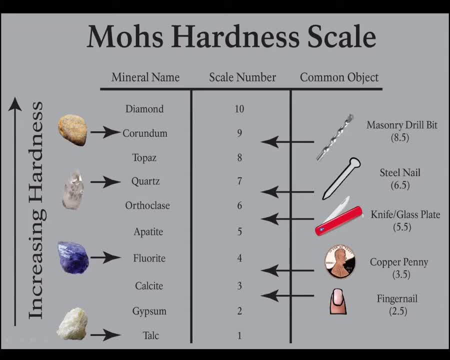 a hardness. some are soft enough to be scratched by your fingernail and some are nearly hard as diamonds. Diamond happens to be the hardest mineral. The Mohs scale of mineral hardness is a scale that ranges from one to ten that is used when identifying minerals with one. 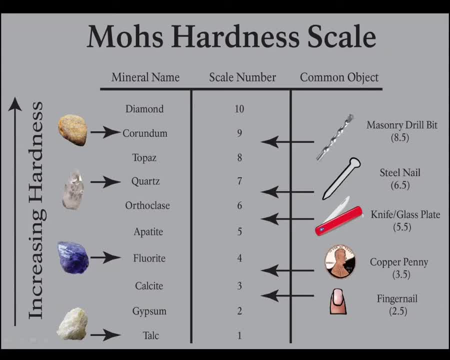 being the softest and ten being the hardest. As you can see, your mineral identification kit is equipped with items necessary for testing hardness. The first test is called a mineral. The fingernail has a hardness of 2.5, so if you can scratch the mineral with your fingernail, 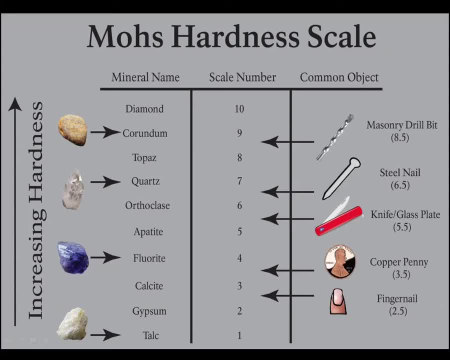 its hardness is less than 2.5.. If you can't scratch the mineral with your fingernail but can scratch it with a copper penny, the hardness is less than 3.5, but greater than 2.5.. You get the picture. 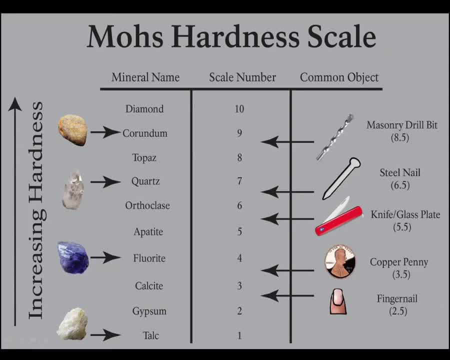 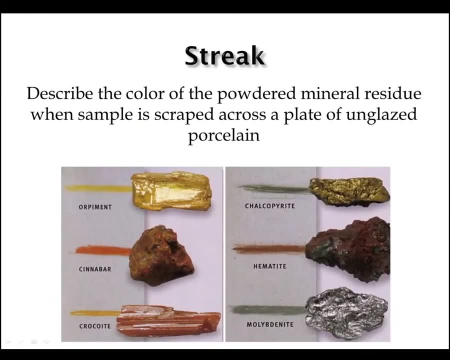 Hardness is one of, if not the most important test to perform on every mineral you attempt to identify. A mineral streak refers to the color of the powdered mineral residue when a sample is scraped across a plate of unglazed porcelain. Unlike the color of a mineral, the color of the streak is relatively consistent. 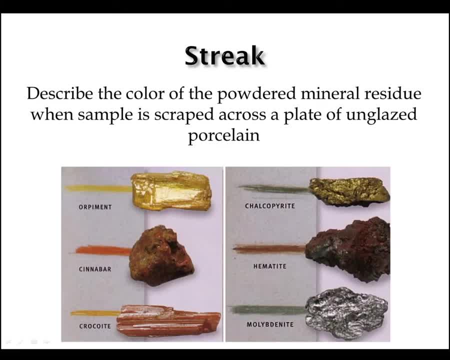 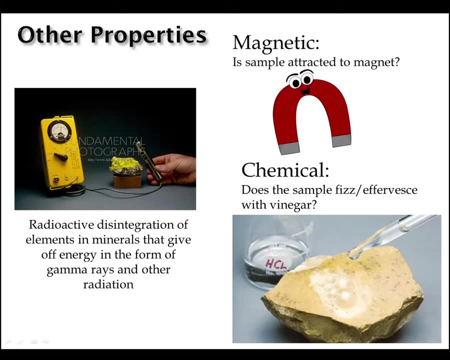 If a mineral has no streak, it is noted as white or colorless. The streak test is also very important when identifying minerals. Other mineral properties that can be tested include radioactivity, magnetism and reaction with acid. A Geiger counter can measure the amount of radiation coming off of a sample. 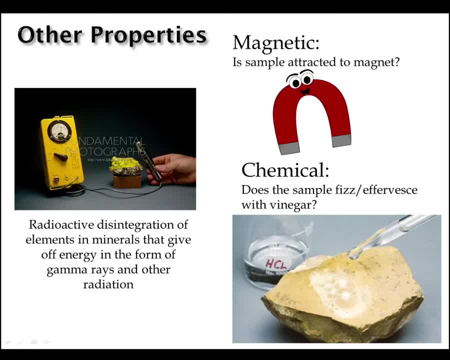 This test is used, but not commonly. However, testing whether the mineral is attracted to a magnet and if the mineral reacts with acid when it is put onto its surface are two tests that should always- always- be performed. Many mineral tests are not always effective. 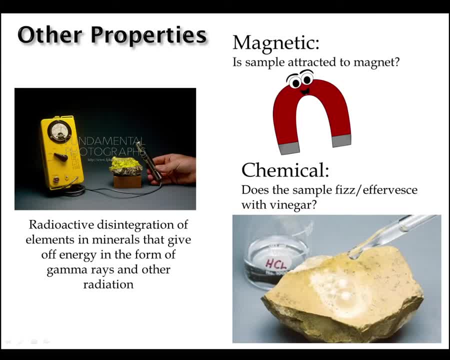 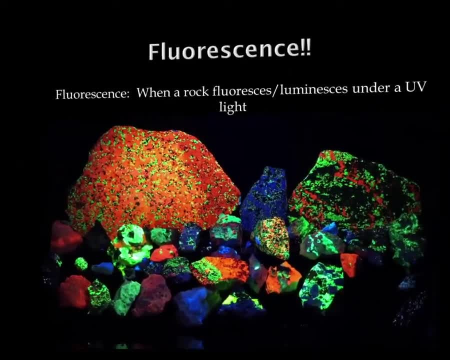 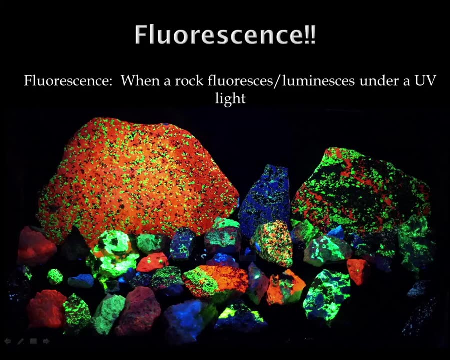 Many people get hung up when trying to identify a mineral by not completing these two quick and simple tests. Fluorescence is one of the most spectacular properties to see in a mineral. Certain minerals are made of elements that absorb ultraviolet light and get excited, or 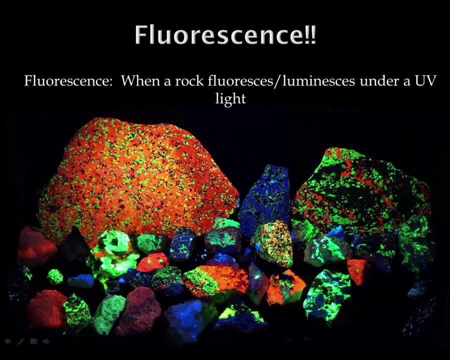 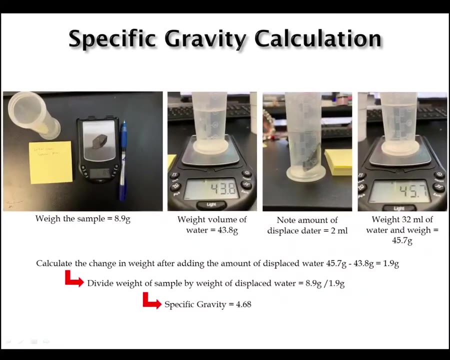 jump up to a higher energy state, as they do When they calm down or drop to a lower energy state, light is emitted and they exhibit fluorescence. The display of fluorescence can help when identifying minerals Specific Gravity: To get the exact specific gravity of a sample. 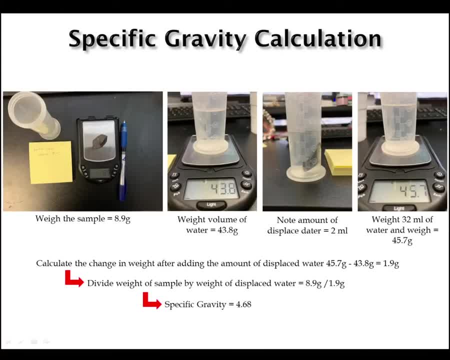 you need a sample that has no other minerals present- which doesn't really happen very often- and some high-end equipment. But to get a general idea of what the specific gravity is, you can perform the test yourself. Refer back to this screen if you would like to give this measurement a try. 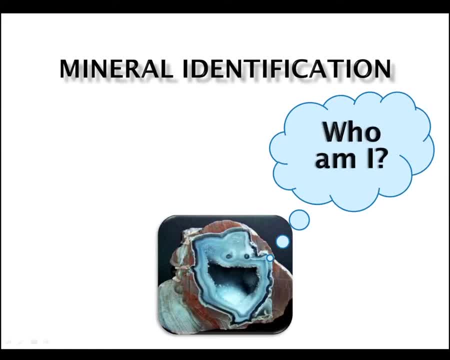 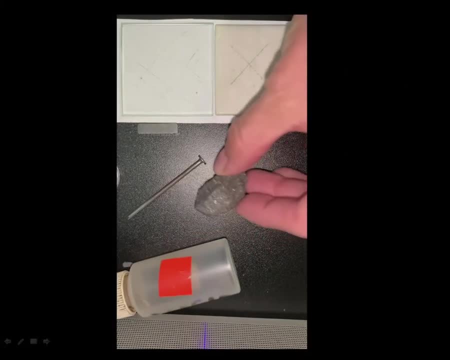 Now it's time for some mineral identification. We will now look at and identify two minerals, So let's get started. Here is our first mineral specimen. We can see it looks metallic and there aren't any definite crystals visible. with the tools we are using, 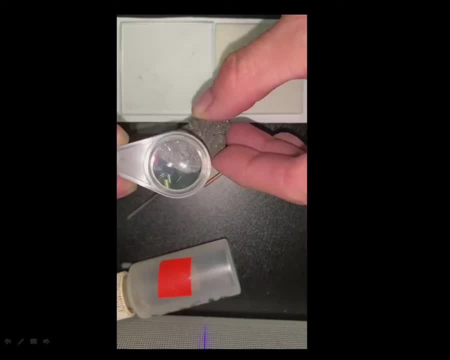 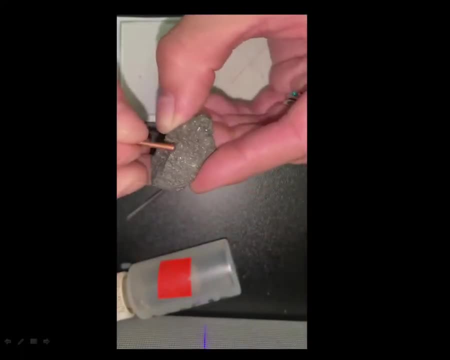 So this is a massive mineral aggregate. We will first see if the mineral can be scratched by a fingernail, Which it cannot. Next, we will try the copper. If you look carefully, you can see that the copper is left on the rock. 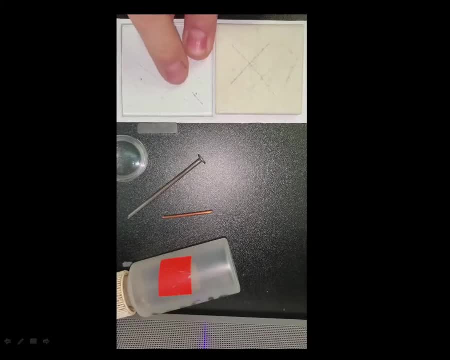 So we will move up on the hardness scale and see if our sample will scratch glass, Which it does. So the hardness is greater than 5.5.. Don't be afraid to really put some pressure on the glass plate to see if a mineral will. 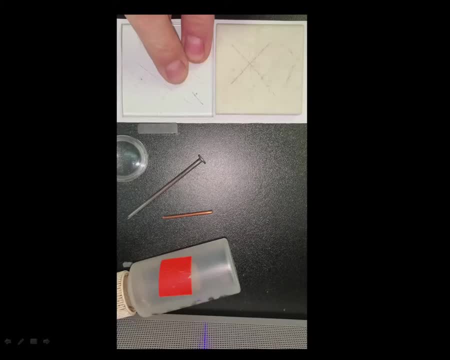 scratch or not. I did not show the nail in this video because it was really hard to see, but it does scratch the mineral, so the hardness is less than 6.5.. Now we will scrape the mineral across the white plate and we can clearly see the streak. 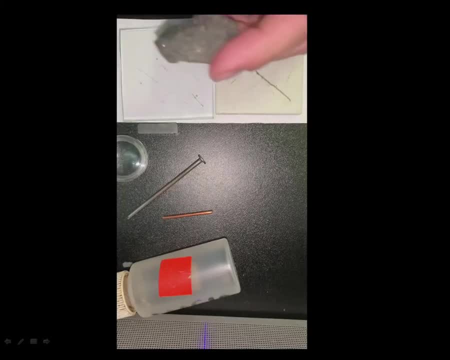 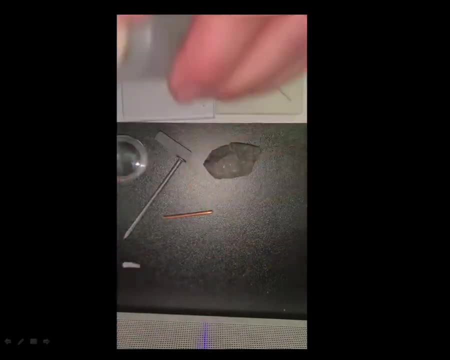 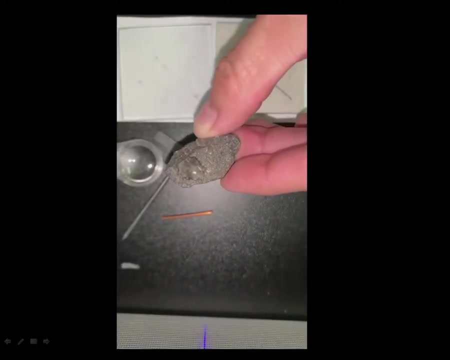 is black. Now it's time for the magnet. Yes, this mineral is very magnetic. Next we will test with some acid. We can see a reaction, but when we thin the acid out, it is easy to see that the sites where the reaction is. 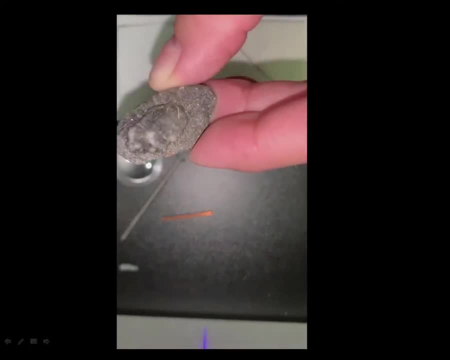 taking place correspond with some white spots that are in the sample. This is not the mineral we are trying to identify, However. calcite is a mineral that reacts vigorously with acid, so it is probably a safe assumption that the white spots in this sample are calcite. 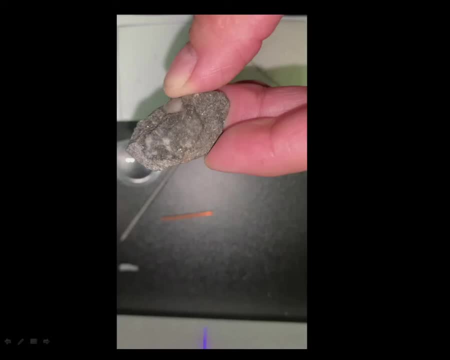 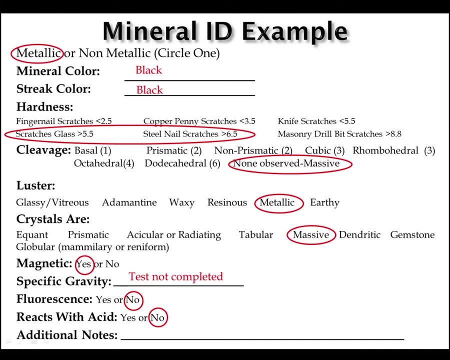 But what are they with? Let's continue. When identifying rocks and minerals, it is good practice To write down your observations and results from the test you perform, also known as the data. Here is our data. We will use this data in the next phase of our mineral identification exercise and you 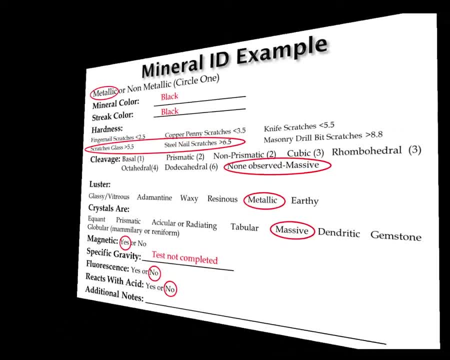 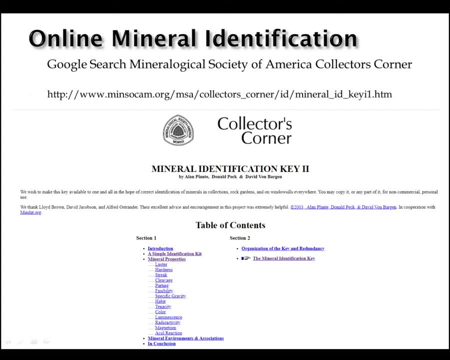 can refer back to this later. if needed. We will use the Mineralogical Society of America's Mineral Identification Key, which ultimately links with a very large online database, MnDATorg, Which we will look at in a few minutes. We will click on the link to the Mineral Identification Key. 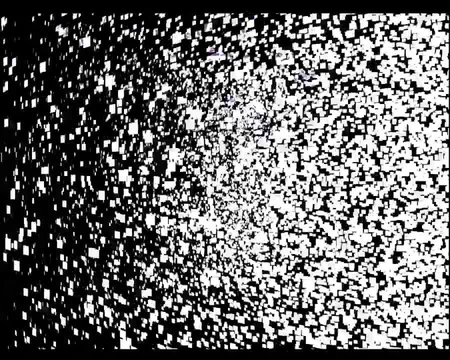 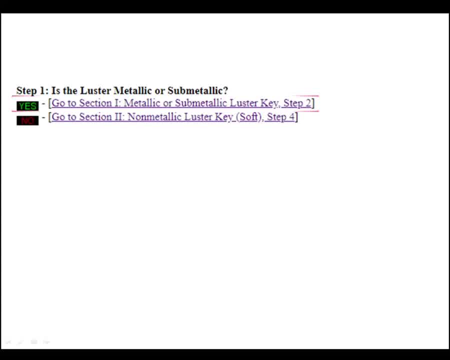 We arrive at the first question: Is the lustre metallic or submetallic? Our mineral was metallic, so we will choose yes. Next, will the mineral leave a mark on paper or is the hardness less than 2.5? No, 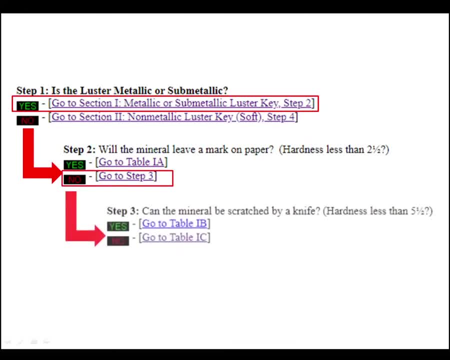 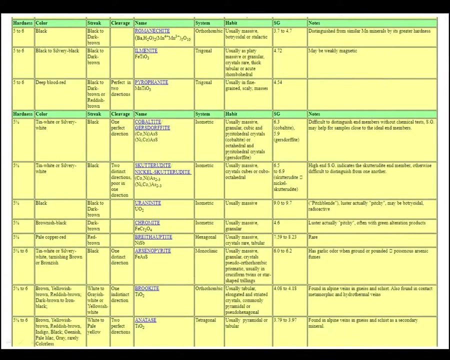 Our mineral would tear up some paper. Next, can the mineral be scratched by a knife? Though we did not test with a knife, we can select no, because it scratched glass, So a knife could not have scratched it. So when we select no, we are redirected to this intimidating table. 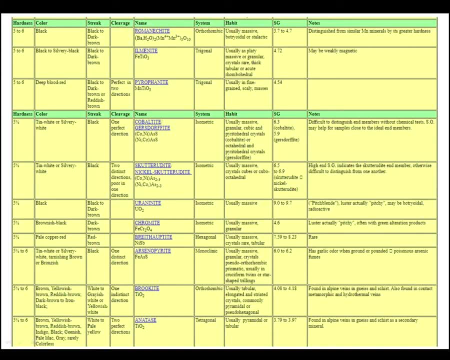 But don't run away. It's really not that bad. We can eliminate most of these minerals very quickly. First, the hardness has to be greater than 5.5. So let's eliminate all of the minerals with a hardness of 5.5.. 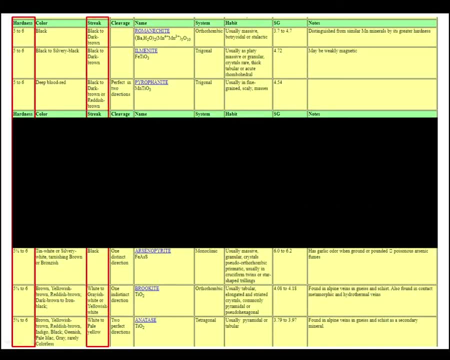 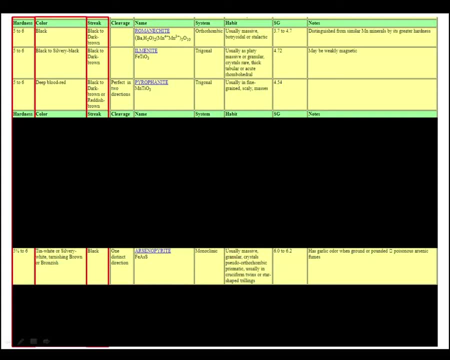 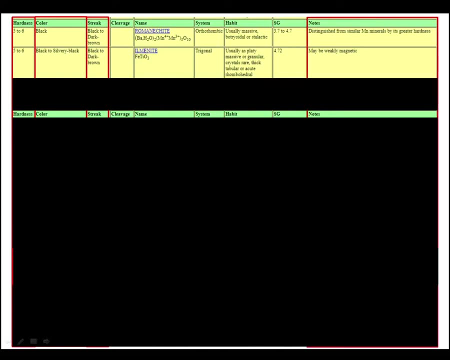 Next, let's look at the color of the streak. If it isn't black, it's gone. Moving on, We will get rid of any mineral that doesn't have black as a mineral color listed. And finally, we will look at the notes. 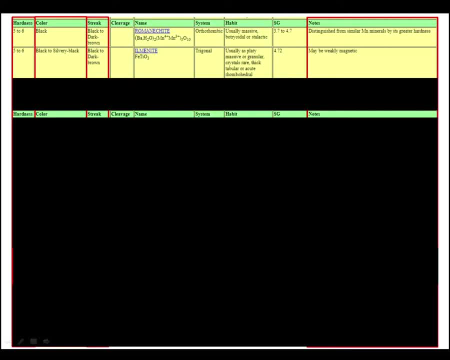 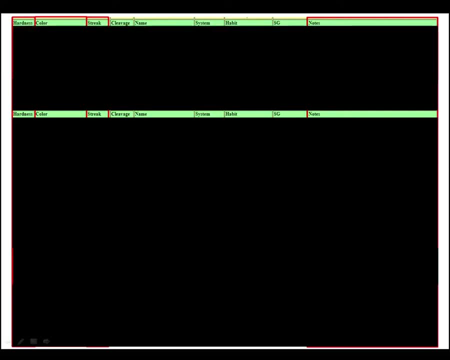 There is only one mineral left that might fit the bill. We will look at the notes. There is only one mineral left that might fit the bill, But it is only weakly magnetic. So all of these minerals are eliminated and we scroll down. 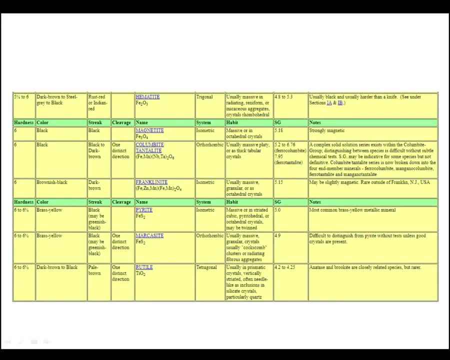 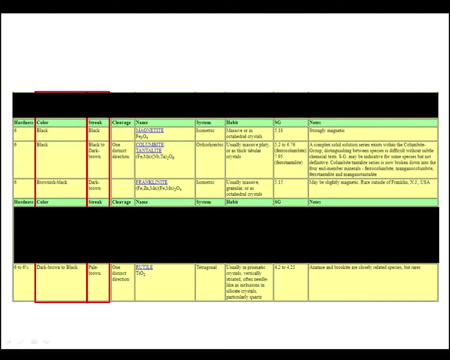 All of these minerals have a hardness that fits our sample. So let's look at the streak and eliminate the one that's not black. Next, let's move to color and eliminate any mineral that doesn't have black as a mineral color listed. Now, since we are towards the end of our list. 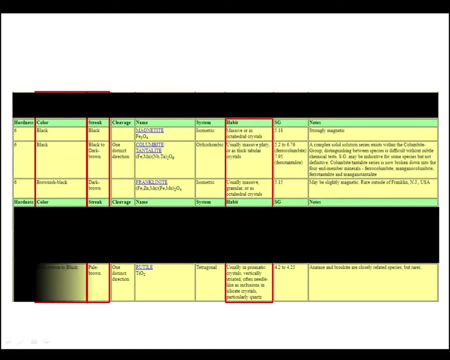 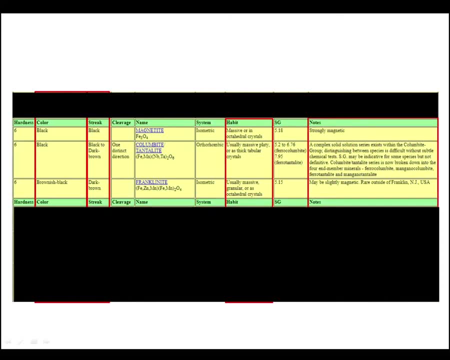 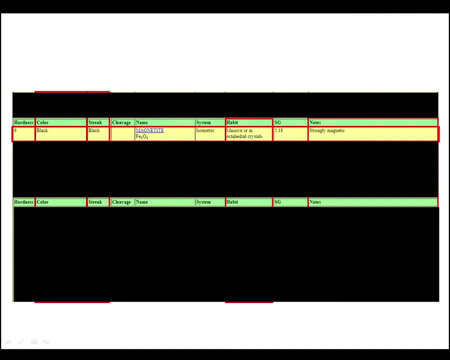 Let's look at habit and get rid of any that don't occur as massive mineral aggregates. And finally, we will look at the notes of the remaining candidates And we can see that there is only one that mentions being strongly magnetic And the mineral is magnetite. 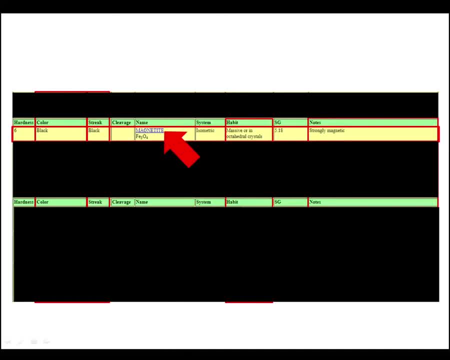 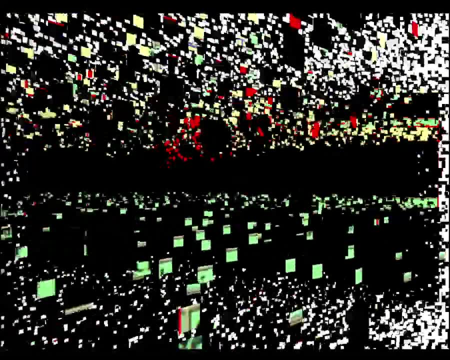 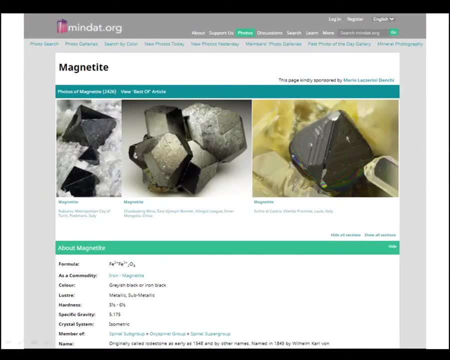 This sounds like our culprit. If we click on the mineral name, which is a hyperlink, it will take us to another page. This is Mendatorg, a large online database for minerals. We are taken directly to the magnetite page where you can view photos of the mineral along. 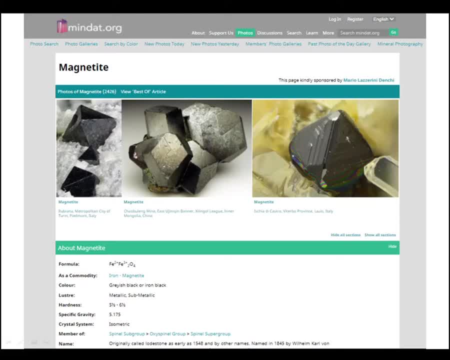 with a wealth of other information. If the results aren't what you expected, it is always wise to go back and observe or test some more. Also, if you get to a result that is suiting, but one of your observations or tests didn't, 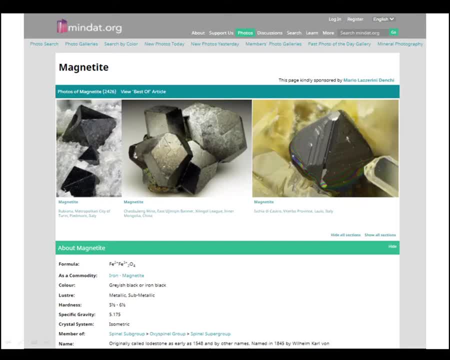 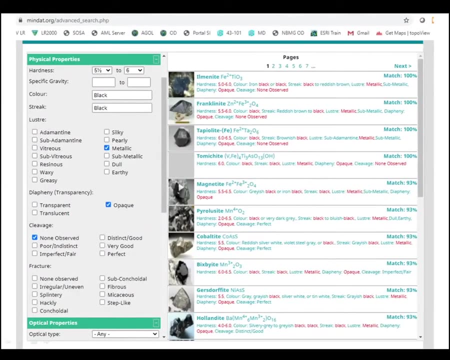 quite match up. Go back and assess the test or observation to figure out what may have went wrong. This is where you learn and grow. as a mineral identifying aficionado, Mendatorg also has a form that can be utilized to identify minerals. There are lots of advanced options, but fill in the data you have and review the minerals. 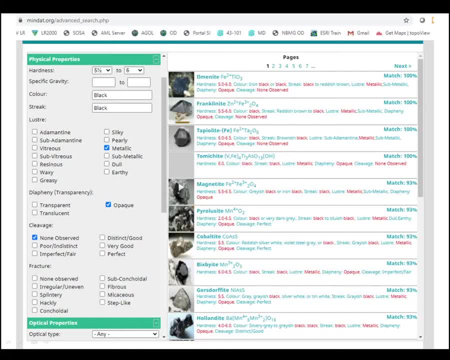 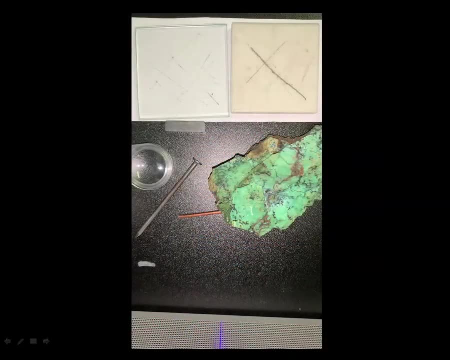 that show up. You can see after entering the data we have for our sample. Magnetite is a 93% magnetite. If there was an option for magnetic, I'm sure that number would rise to 100.. Let's work through one more mineral together. 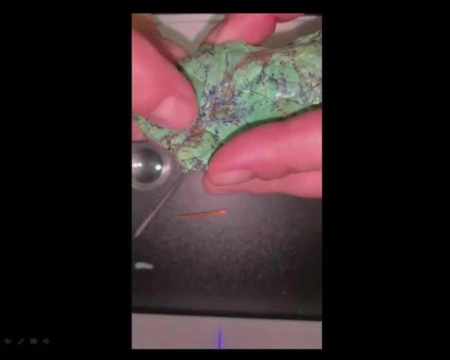 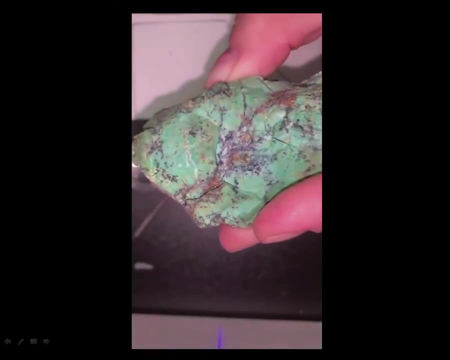 First let's see how hard it is. It can't be scratched with a fingernail, but it can very easily be scratched with a piece of copper. so the hardness is greater than 2.5 and less than 3.5.. 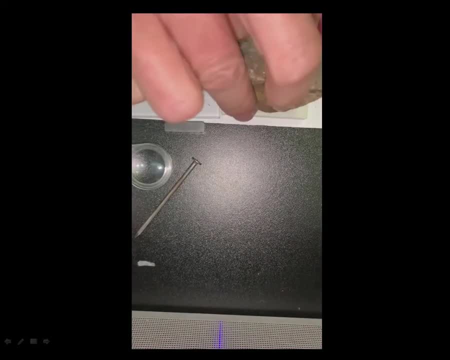 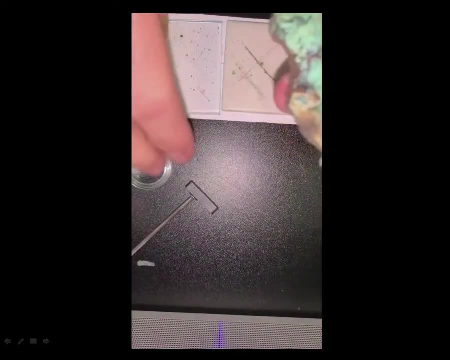 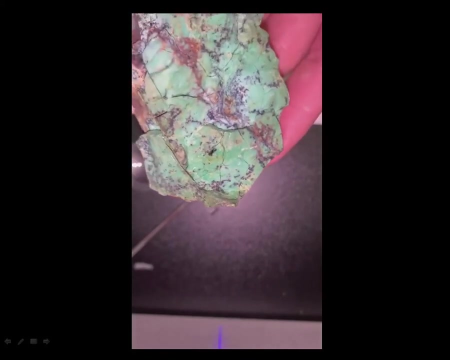 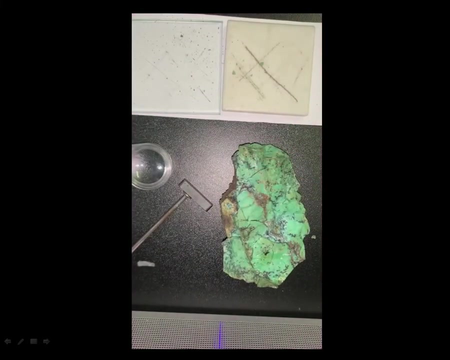 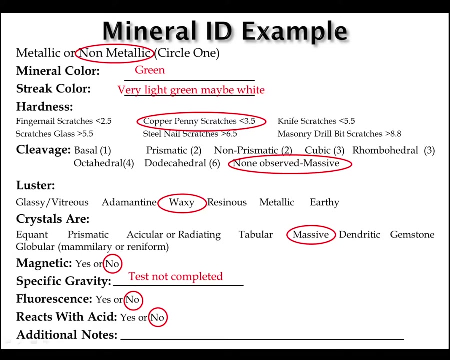 The streak is hard to see, but it is white or very light green. 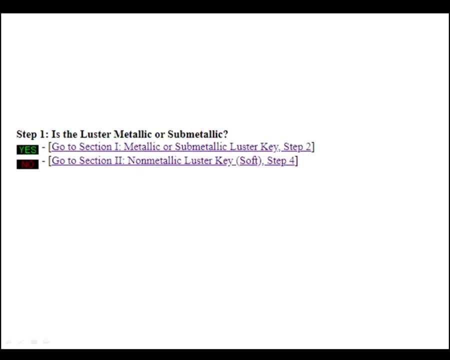 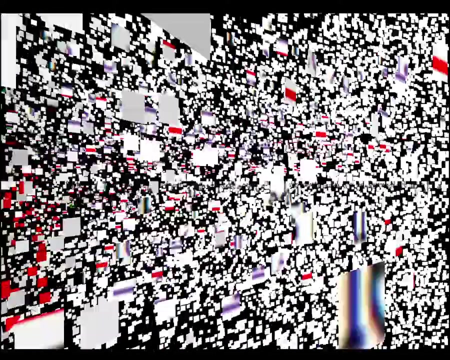 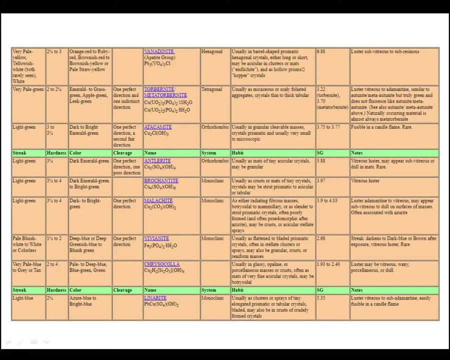 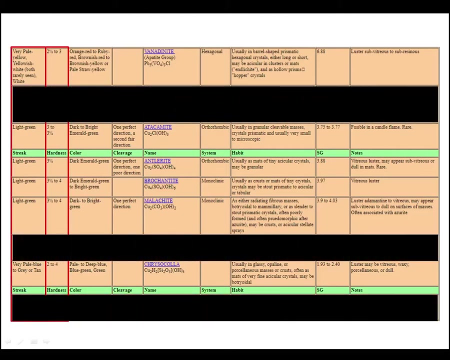 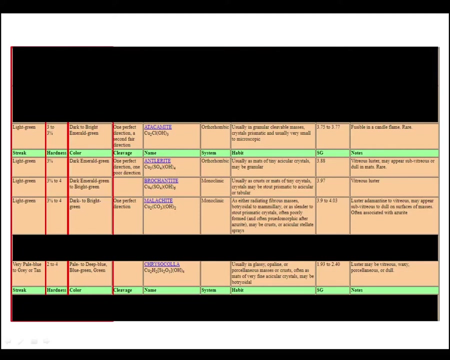 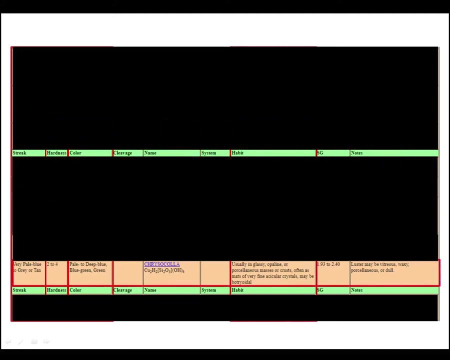 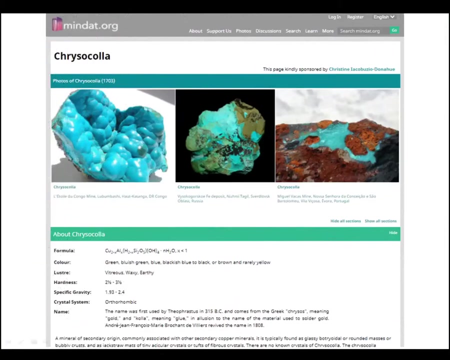 And we can see that the middle photo pretty closely resembles our specimen. I would feel very comfortable calling this mineral chrysocolla. 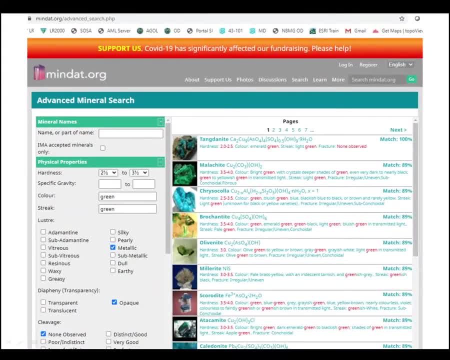 Looking again at the mi undat dot org advanced mineral search form and filling in our data, we can see chrysocolla is a pretty close match, being third on the list. Malachite is much brighter, green and vitreous than our mineral. 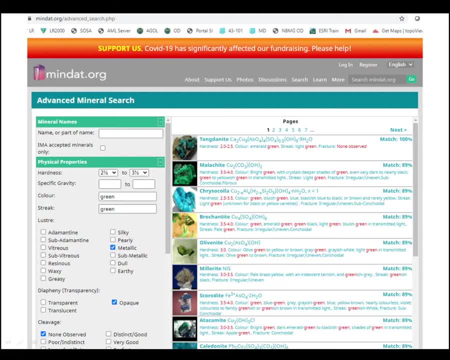 and tangdonite is too soft. One last thing I would like to say on mineral identification: Always remember the law of least astonishment, Unless you have been to some obscure place in search of some obscure mineral. if you identify a specimen and end up on a mineral, that is. 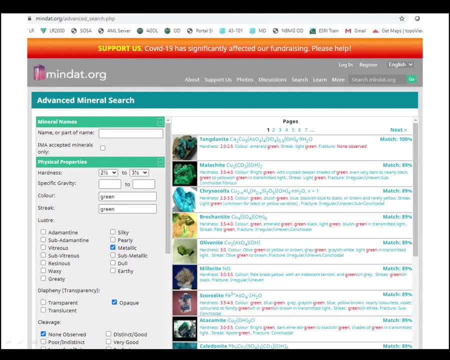 incredibly rare or only found in one place of the world, it is probably not the mineral you have in your hand. With time, you will become familiar with the common varieties of minerals. Also, if you happen to land on an obscure mineral species, identification sources almost always.